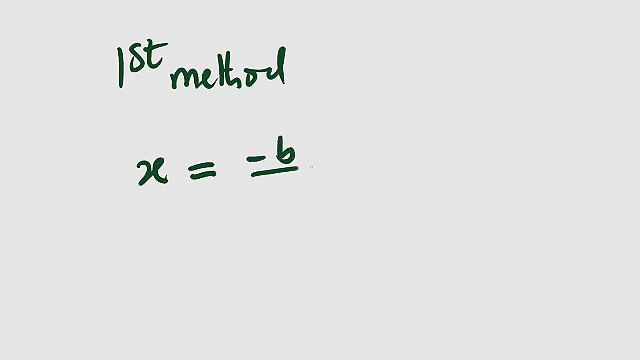 x at that point is equal to minus b divided by 2a, And what is b? b is always the coefficient of x, while a is the coefficient of x squared. So this is equal to minus. what is b- b is 2.. 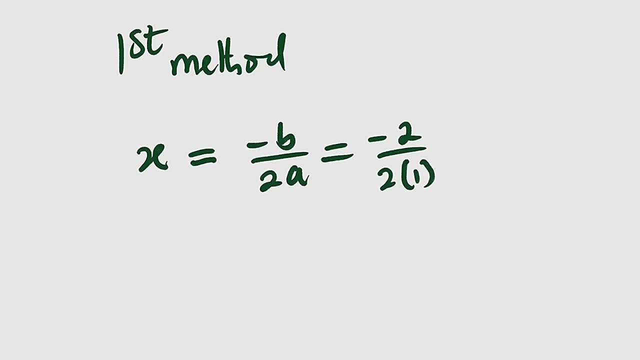 2. 2 times a is 1.. If you simplify this, you shall obtain negative 1. So x is equal to negative 1.. You can also use differential calculus to find this negative 1, because you should know also that at this particular point the first derivative is equal to 0.. 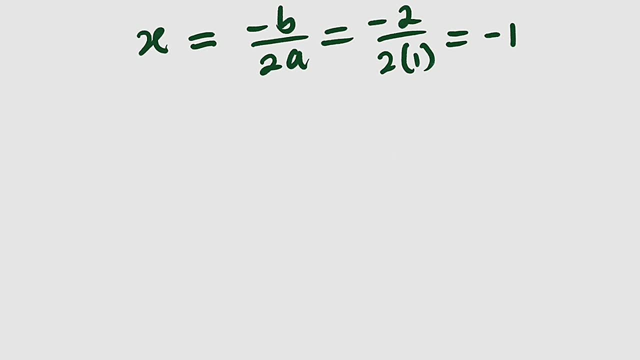 So we can differentiate that function and set it to be equal to 0.. Remember, our function is f of x equal to x squared plus 2x minus 3.. If we differentiate this function, f, prime of x equal to the derivative of this will give us what. 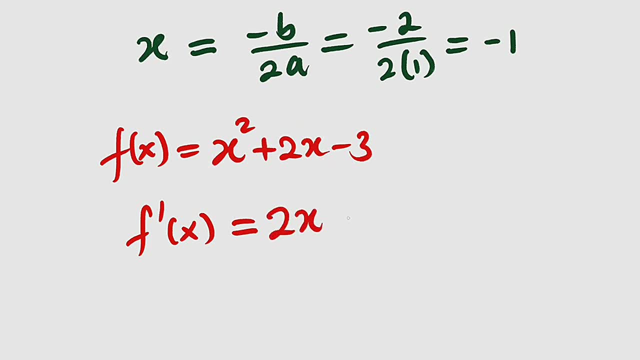 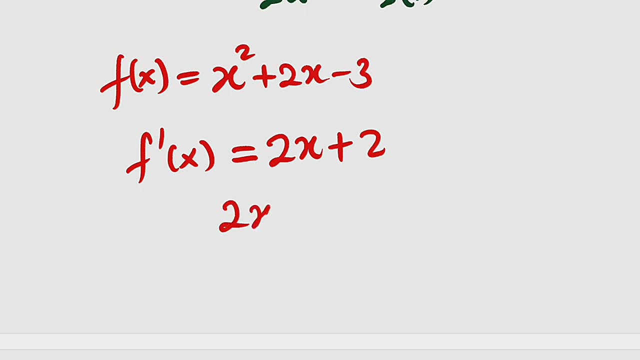 2x, And the derivative of this will give us 2,. right, That is plus 2.. Derivative of constant is 0. So if we set this to be equal to 0, that is 2x plus 2 equal to 0.. 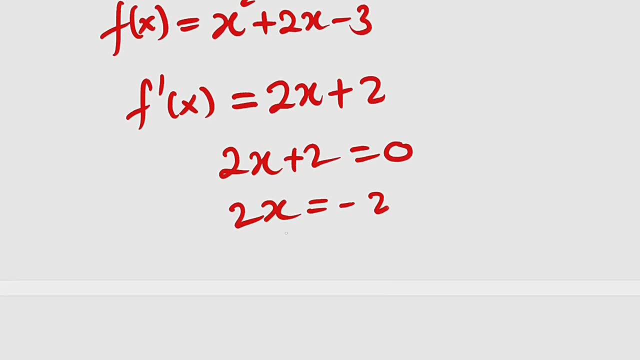 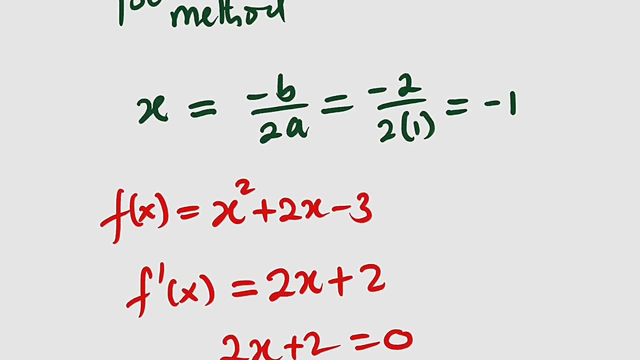 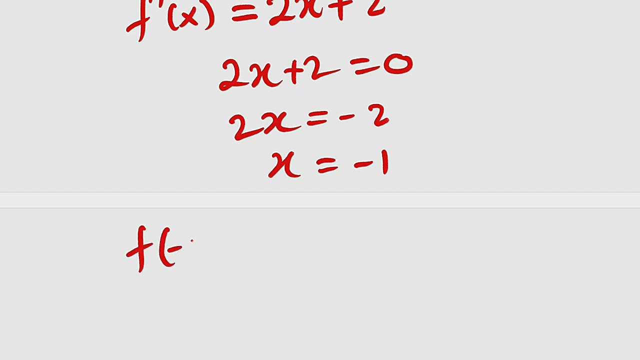 2x equal to negative 2.. Divide both sides by 2, you have x to be equal to negative 1. So, in either case, you are going to, So we are going to substitute it into the main function, that is f of negative 1.. 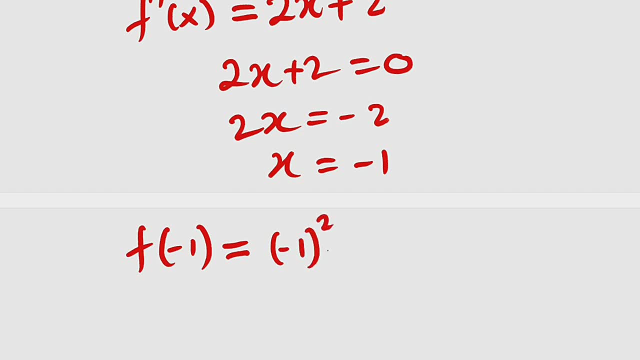 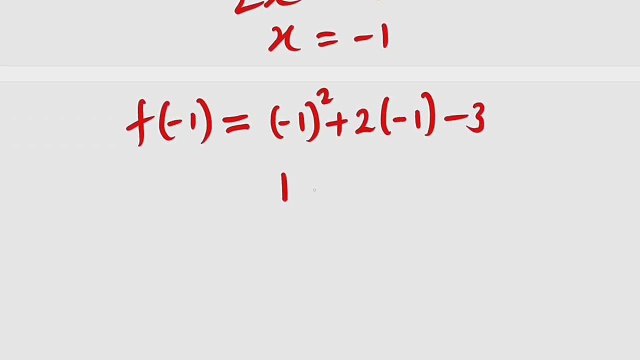 This is equal to x squared, which is negative, 1 squared plus 2x, which is 2 times negative 1, then minus 3.. Negative 1 squared is positive 1.. 2 times negative 1 is minus 2, then minus 3.. 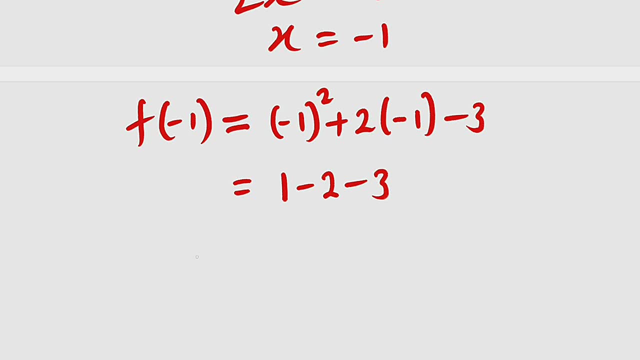 1 minus 2 is minus 1.. Minus 3 is minus 3.. Minus 4.. So this is equal to minus 4.. It means that y at that point is minus 4.. This is the first method. 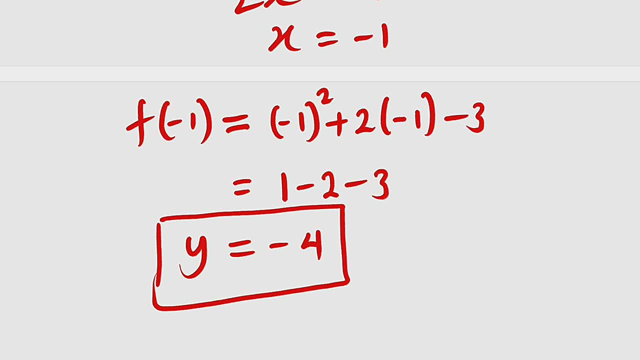 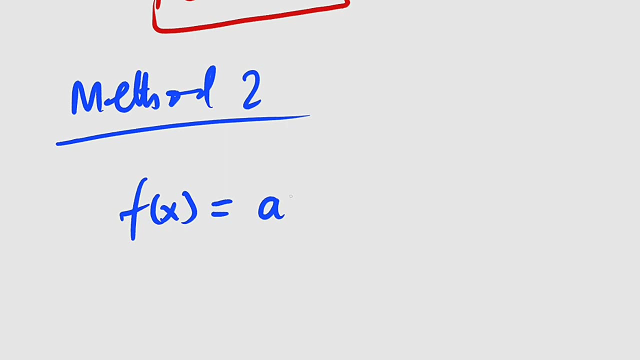 And the second method. I would like to use vertex form of a quadratic function. The vertex form is given as f of x equal to a, which is the leading coefficient. In our case, we have 1 multiplied by x minus h. This h is the value of x at that point, which we obtain here. 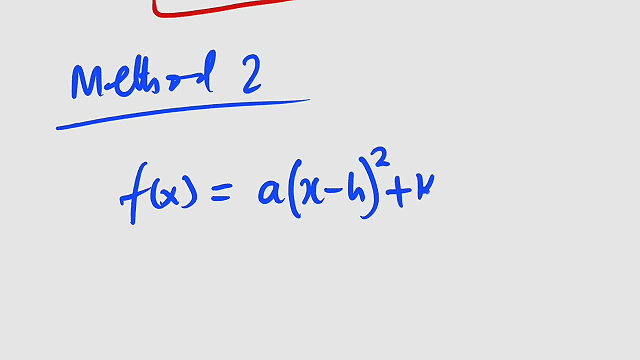 So this is equal to negative 1 squared then plus k. So this particular k is the value of y at that point. So y will be equal to k at that point. So how can we transform our quadratic function in this form? Let me show you. 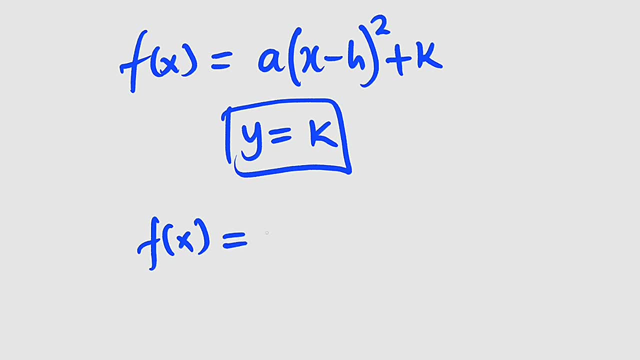 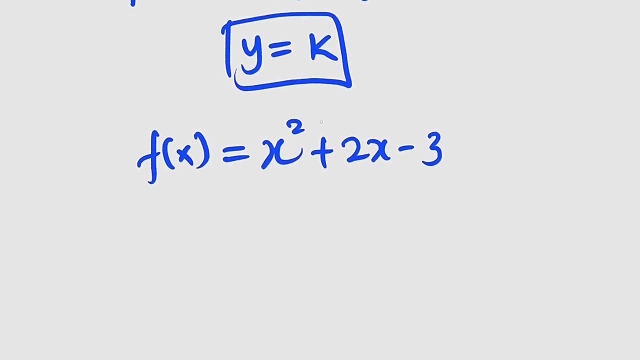 Remember we have f of x equal to x squared plus 2x, then minus 3.. We are going to transform the first two terms into a perfect square quadratic expression. So we have f of x equal to x squared plus 2x. 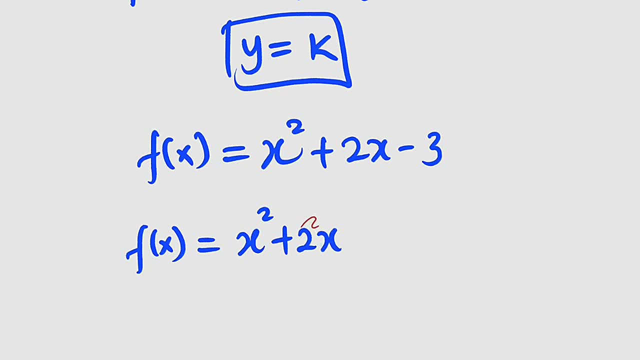 What can we add to these two terms to make it a perfect square? Half of this is 1.. 1 squared is 1.. So if we add 1 here, it is going to be a perfect square. But since we don't have this 1, we are going to take it away. 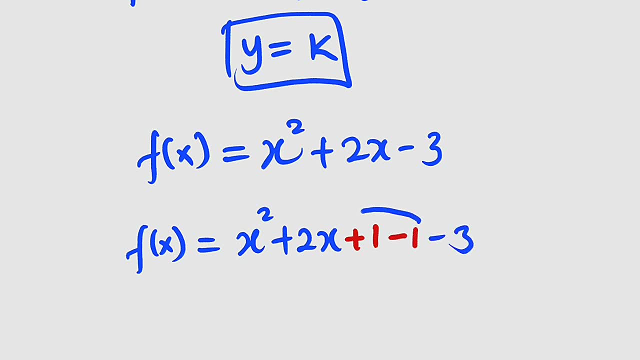 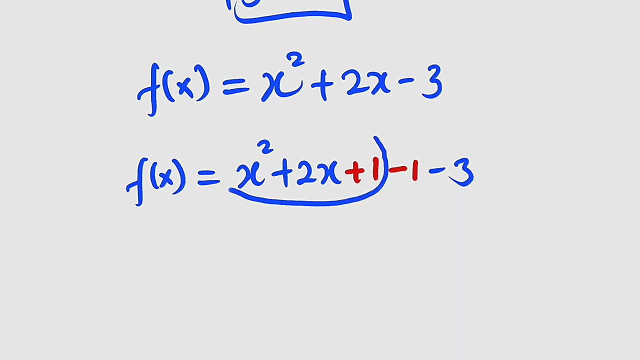 Don't forget to bring negative 3 back. So this is the only thing we have added, which is 0.. 1 minus 1 is 0.. So we have not added anything. The purpose is just to make these first three terms perfect squared. 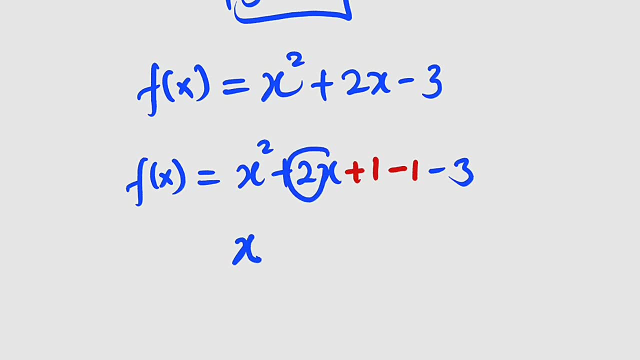 And to factorize it, you take x here without power, then half the coefficient of x, which is 1.. Then you square all. Don't forget, we still have what Minus 1, minus 3, which is minus 4.. 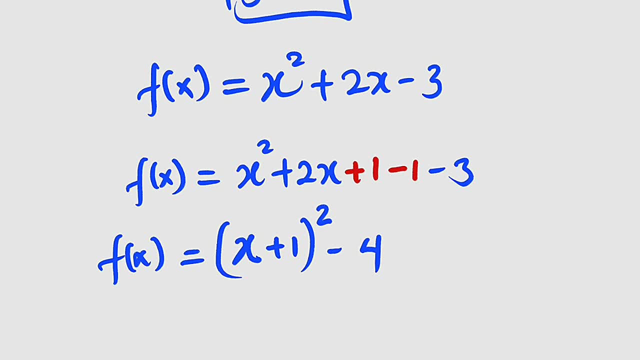 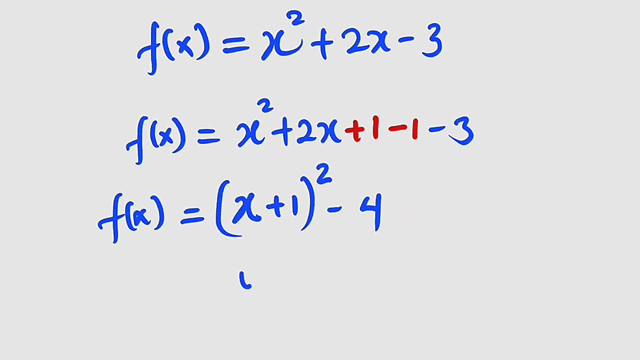 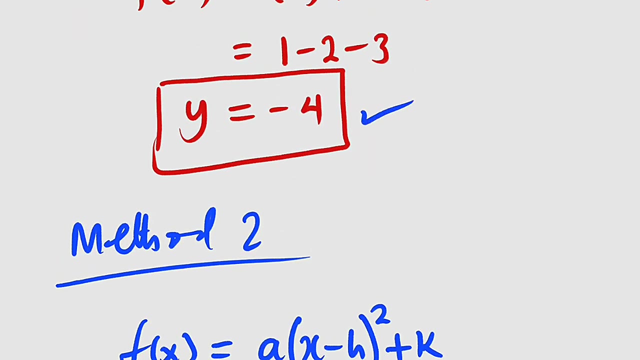 So this is our f of x in vertex form. Remember I told you k is what? The minimum value. Therefore, we are going to consider negative 4.. y equal to negative 4.. The same thing You know previously, we obtained negative 4.. 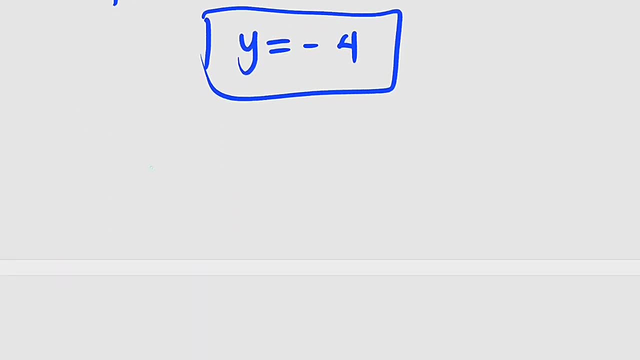 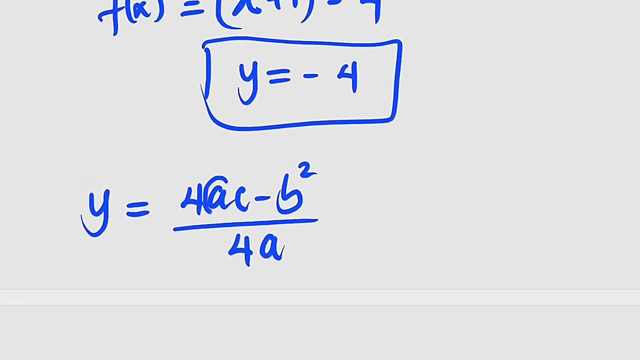 Then the last method. I would like to use formula y, equal to 4ac minus b squared divided by 4a. If you simplify this, you shall obtain this negative 4.. So let's substitute: a is the coefficient of x squared. 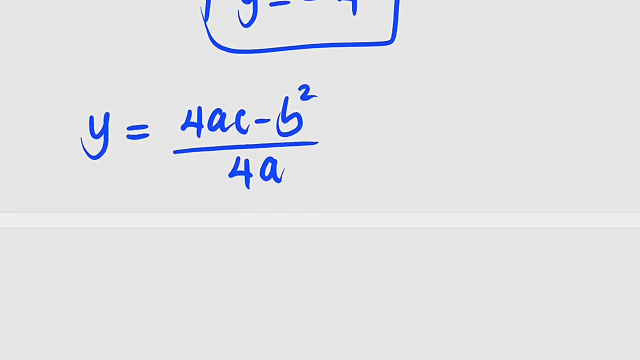 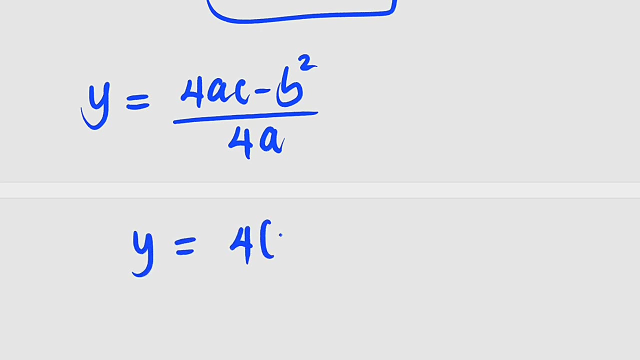 c is the constant which we have here as minus, Minus 3, right, And b is the coefficient of x, which is 2.. So let's substitute them. y is equal to 4 times a is 1.. c is negative 3.. 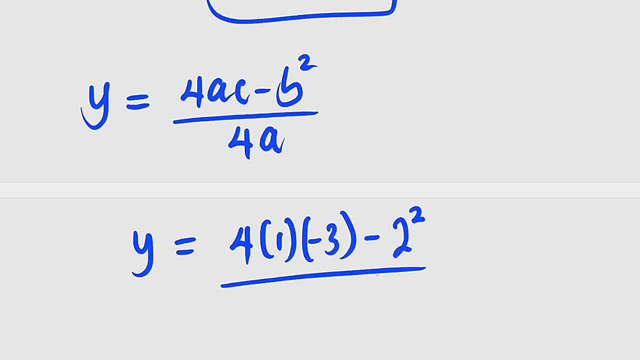 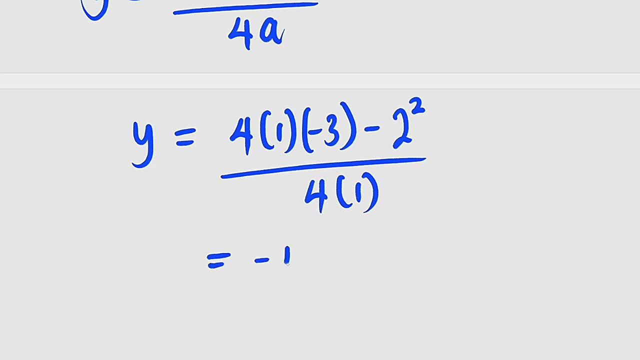 Minus b is what? 2.. So we square 2.. Divide by 4 times a, which is 1.. 4 times 1 times negative 3, will give us negative 12.. Minus 2, squared, is 4..